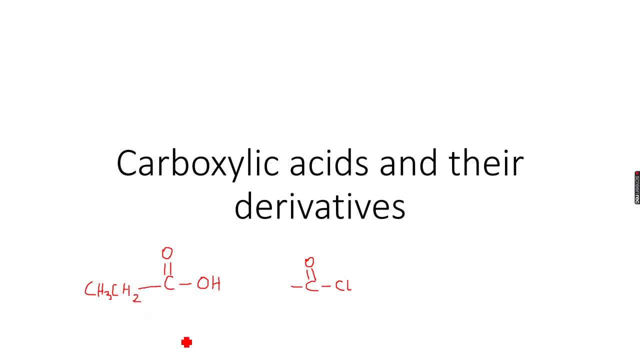 I have. this is: this is called propanoic acid overweight, because we have three carbon atoms in the main chain and group a propanoic acid. so it's acid because of the carboxylic acid group. so it becomes P R O P A O N. so this becomes propanoic acid. and this, if we attach the 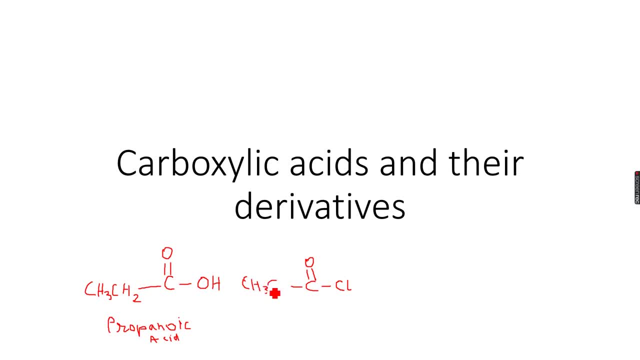 same CH3, CH2 group over here. then this becomes propanoil chloride, so the name is different. you have to know the naming. we have the same prop because three carbon atoms in the main chain and instead of a NOIC, which is here, we have a NOIL, so propanoil chloride. 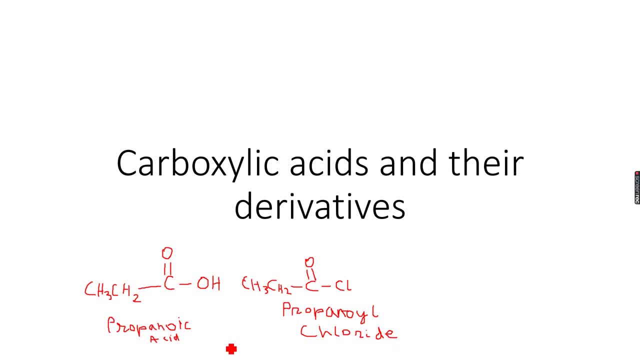 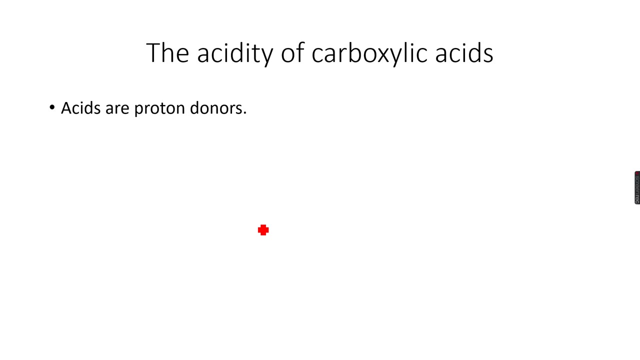 so this is an acyl fluoride, and so we know the naming. now how to name these compounds so we can move further. so the acidity of carboxylic acids. so why are they called acids? because when we, if you will remember, when we studied the Bronsted-Lowry definition of an acid, we know that acids are proton. 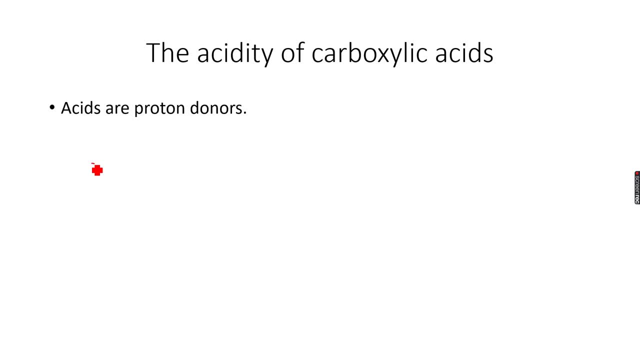 donors. so. So what happens is, let me take the same propanoic acid. when I add it to water I get in a reversible reaction, so I get a carboxylate ion, so this is called the propanoate ion.